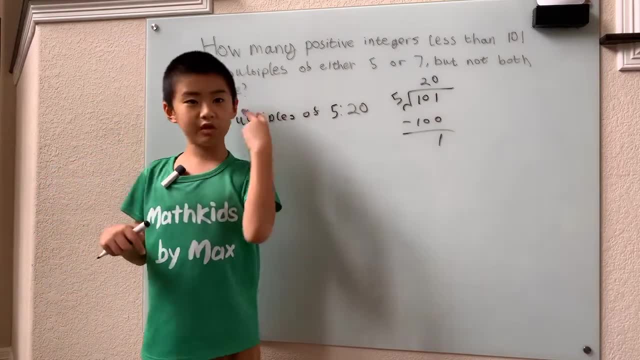 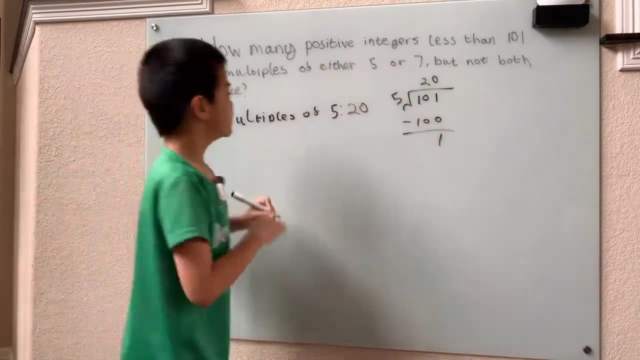 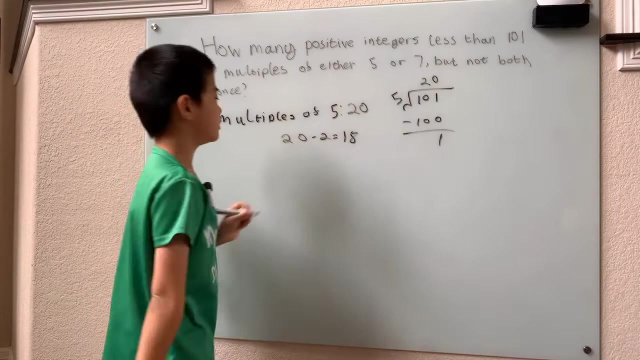 We can't have that. So we can see that there are two special multiples of 5, 35 and 70. But those are multiples of some so we can't count that. So that means there's 20.. There's 20 minus 2, 18- good multiples of 5.. 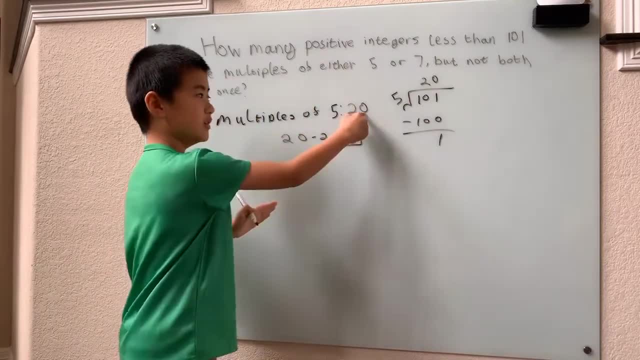 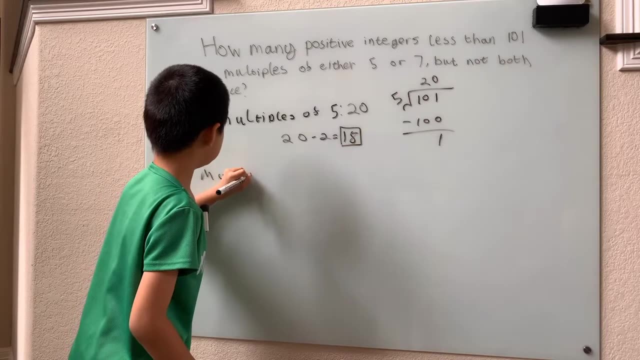 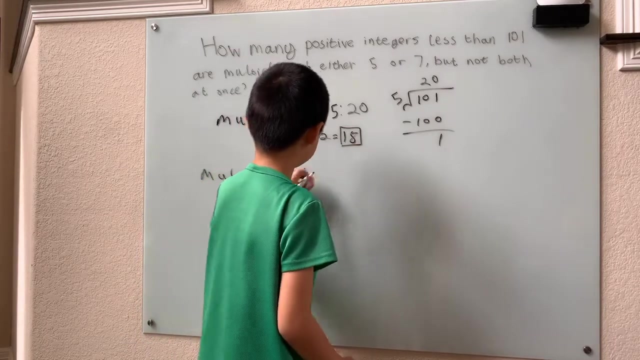 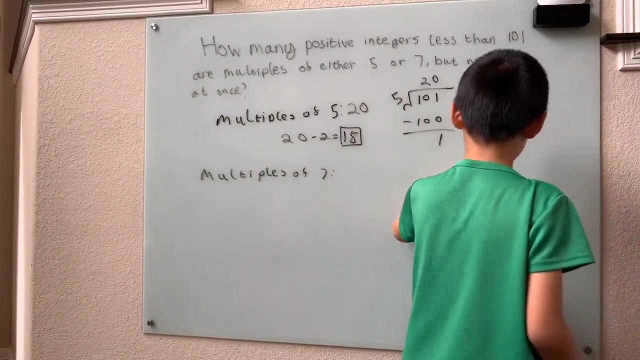 I'm going to go ahead and box that in, so we don't look at 20.. And now the multiples are 7. Multiples of 7.. Now we'll do this with long division too, So we can just easily divide 101 into 7.. 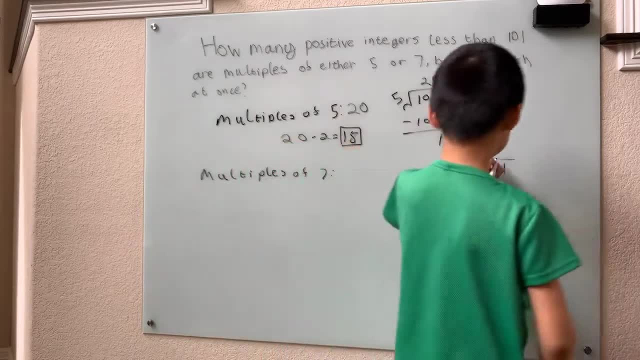 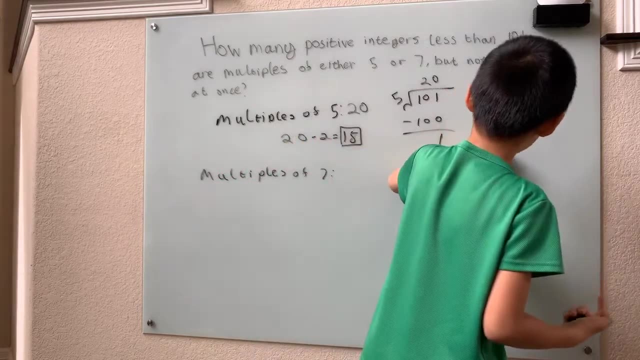 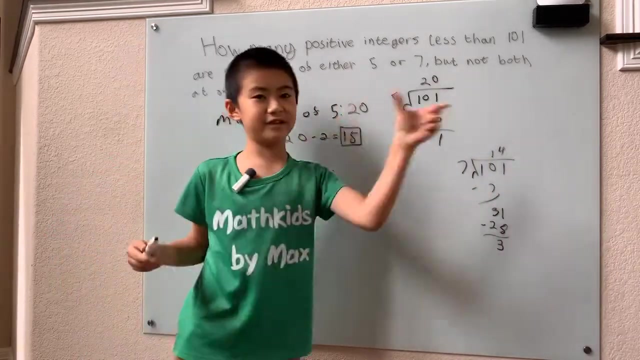 7 goes into 10 once Subtract 7, have 3, drop down to 1. And 7 goes into 31 four times, which will give us a remainder of 3.. Now what that means is we can basically fit in 14 of these little blocks of 7 in 101 before we run out of space. 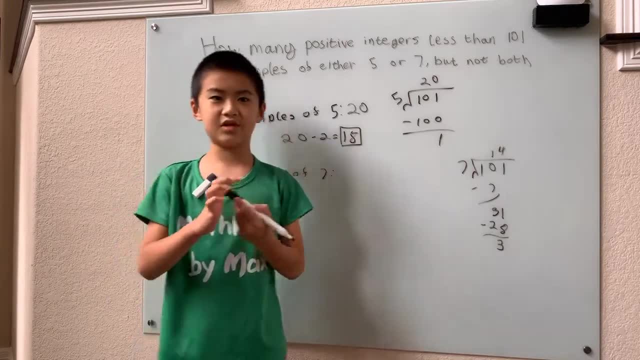 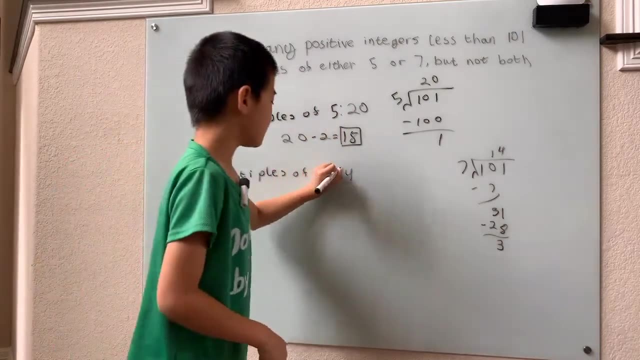 If we run out of space for another block of 7, then we just have to use a block of 3.. So that means there's 14 total multiples of 7.. And well, again according to our rule, there's again two special multiples of 7.. 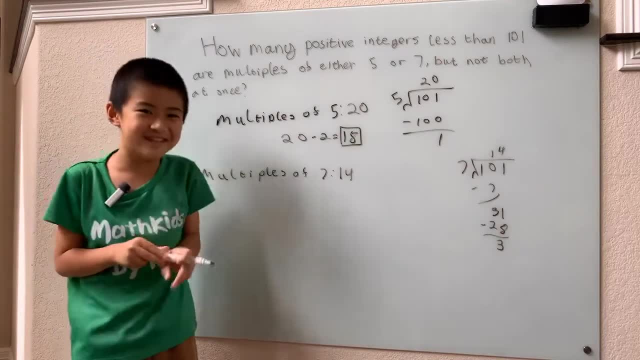 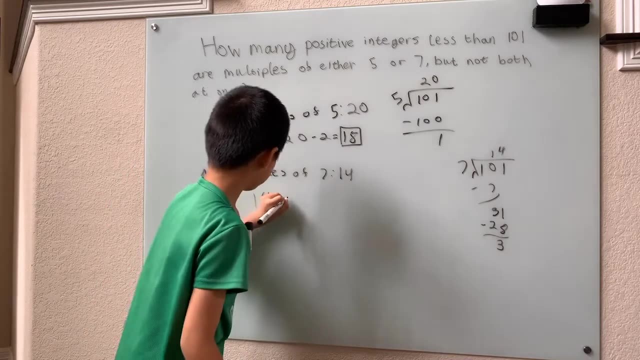 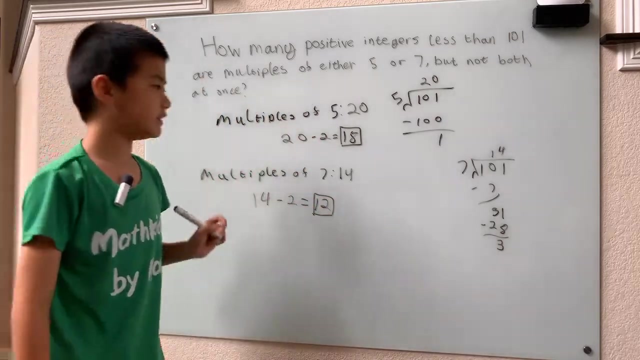 35 and 70. That means they're both multiples of 5.. We can't have that. So that means we just have 14 minus 2. Only 12.. 12 good multiples of 7.. Go ahead, box that in. 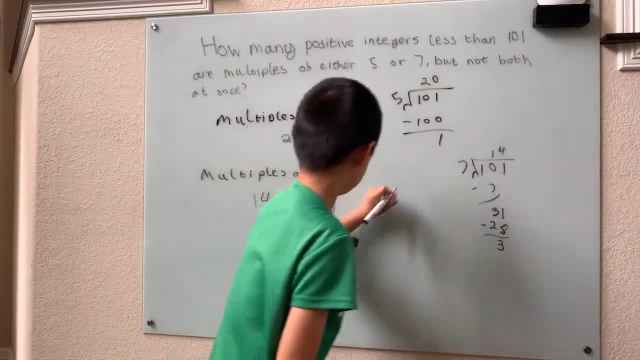 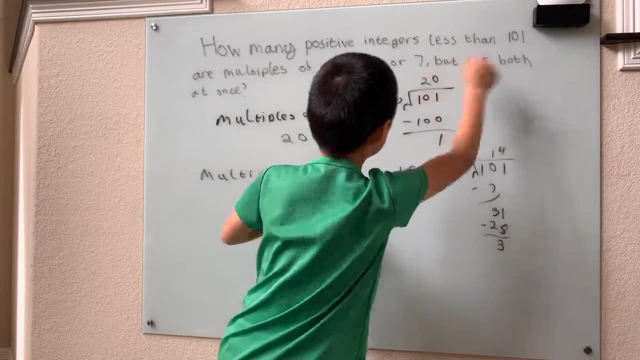 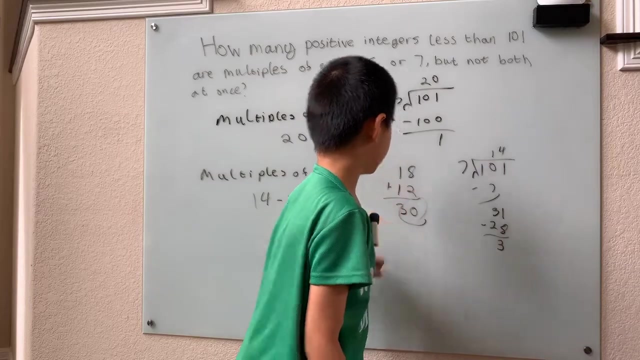 And now we see, finally, since we didn't count anything more than once and we did that, but not both thing, we can just add these two, and when we do add those, we get 3..